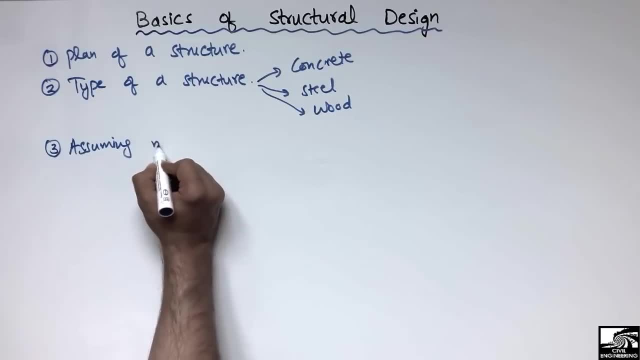 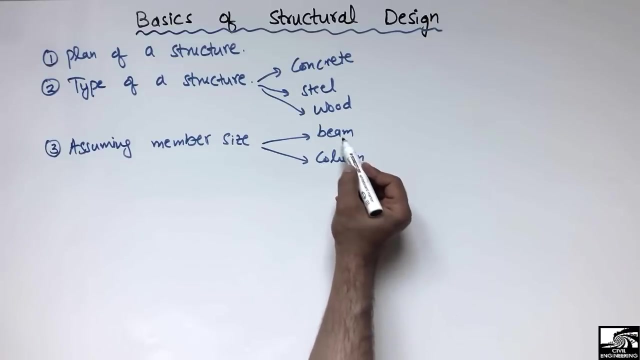 Assuming the member size, This includes the beam size and the column size. These are the two important structure elements. So beam size includes the structure. So beam size includes the structure. It is what should be the beam width and the depth of the beam. 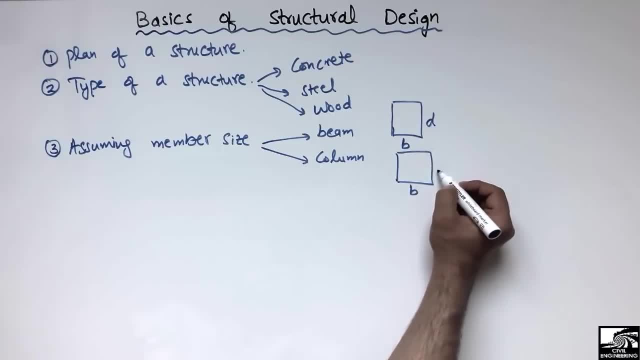 Also the column dimensions, Similarly the column width and the column depth. It is what number we should choose for the dimension of the beam and column, And we should start out designing by choosing the beam dimension and column dimension. So the second step: after choosing the type of a structure, it comes the assuming the structure member size. 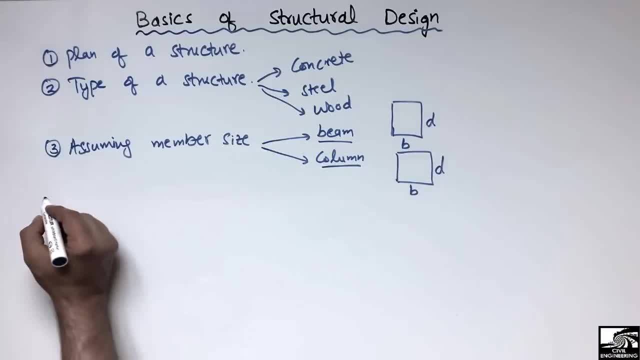 The beam size and the column size. The fourth step is the applying loads on the structure, So the loads applying loads on the structure. It means that you have to take the dead load of the structure or the self weight of the structure, The live load coming on the structure. 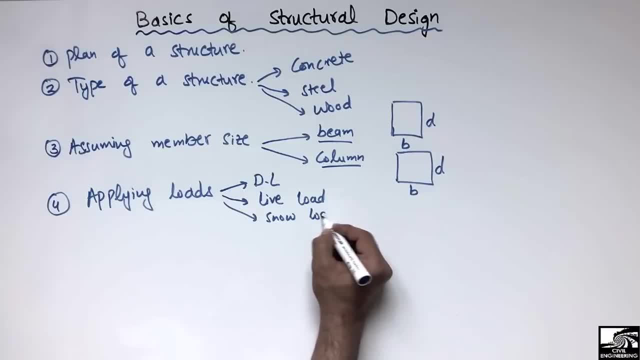 The snow load. If it is in a snow region, then you have to take the snow load. You have to take the wind load on the structure if it is a taller structure. So, depending on where your structure is, you have to take the various kinds of the load and you also have to apply the load combination. 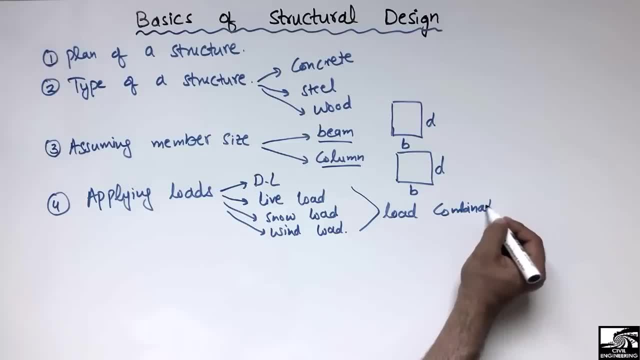 Which one is the worst load combination for your structure and you have to apply the load combination as well. So, after applying the loads, the next step is the structure analysis. In this step we perform the analysis on the structure members. For example, we do the analysis for the shear. 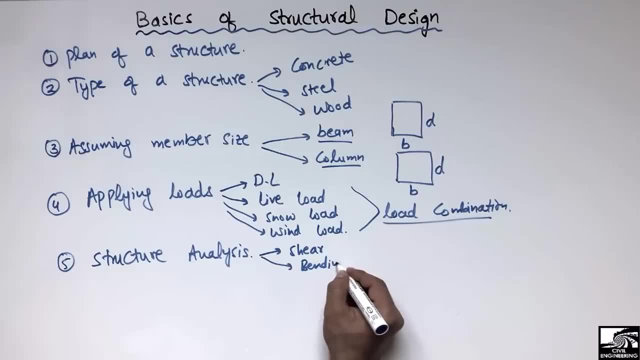 We do the analysis for the bending moment And we get the shear diagrams for the beams and also for the columns and also the bending moment diagram for the beams and columns And we have to check that, how much that how the bending moment changes in our structure. 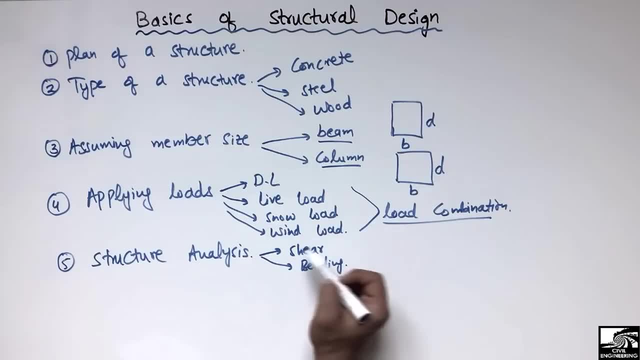 And how the shear varies throughout our structure And according to this we have to design our structure members. So, after analyzing the structure members for the shear force and bending moment and also for the torsion and other type of stresses, So the next step comes is the structural design. 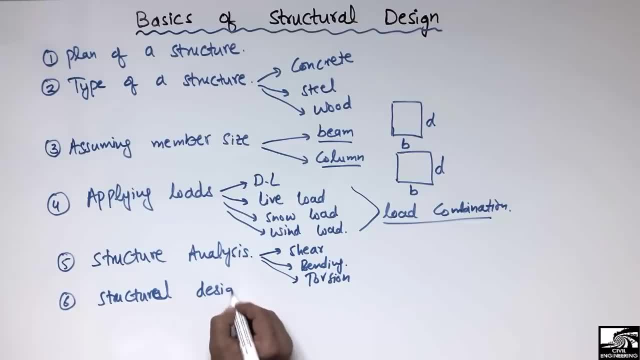 Structural design And this step includes that how much area of friction, How much area of reinforcement we have to provide to resist the various kind of stresses. Area of reinforcement And which type of bar we have to provide, The bar diameter So that we can resist the shear or the bending or the torsion stresses. 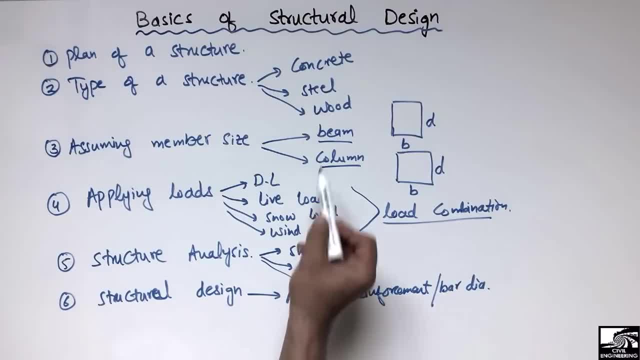 So the sixth step is the design of the structural members: The design of beam, the column, the slab and the footing. So after the structural design, the next step is check for the allowable limits, And this mainly includes the deflection limits. 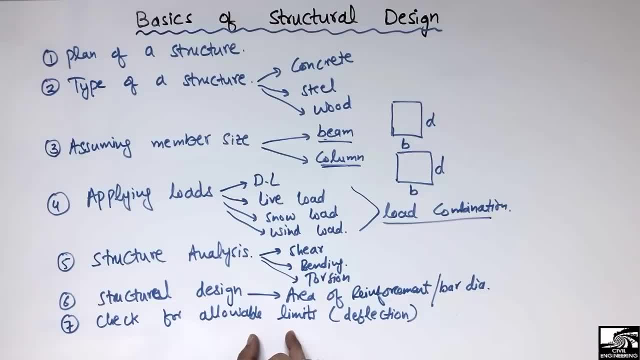 This means that we should calculate our deflection in our structure, members and beams, And we should compare with the limits provided by the different codes, And our beam deflection should be less than the deflection given by the different codes. Otherwise we have to repeat all the steps. 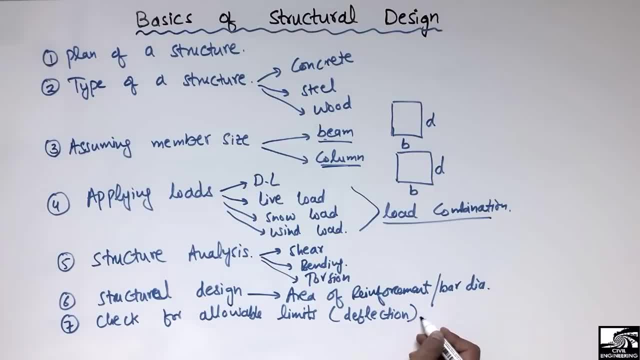 If this step up to this step, if it is satisfied, so it's okay. If it is unsatisfied, if it is not satisfied, then we should again repeat these all steps. Then we should choose again: increase the beam or the column size. 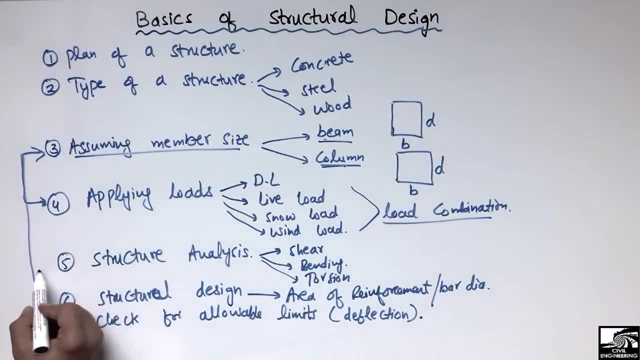 And we should repeat these all steps again, by applying the loads By structure analysis again, By again drawing the shear force and bending moment And again, designing of the beam or column and providing the reinforcement, And again we have to check for the allowable limit. 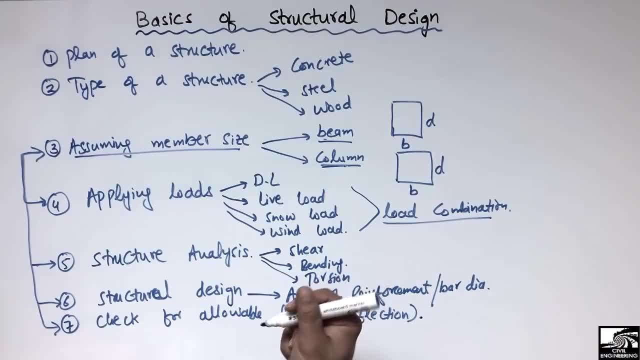 The deflection of the beams, That how much it is higher or lower than the given limits provided by the codes. So, after satisfying the allowable limits, then the next step would be: if this is okay up to this step, Then we have to go to the last step, which is the detailing.